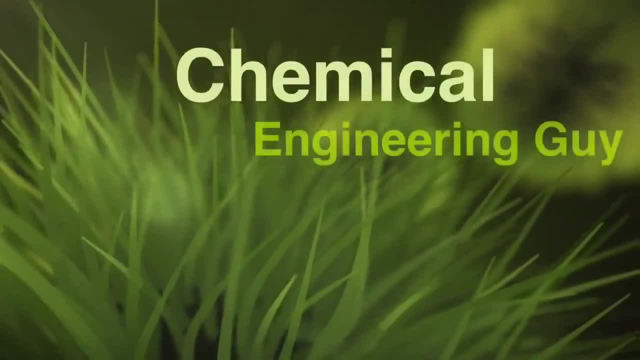 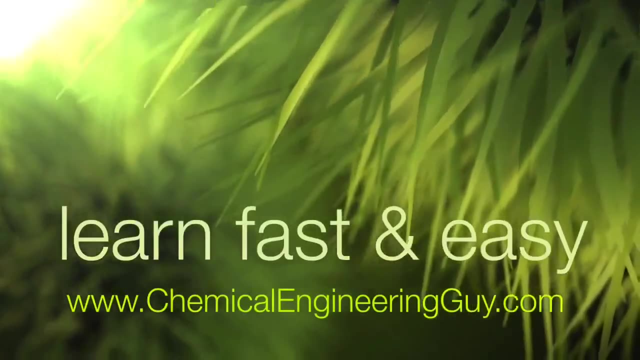 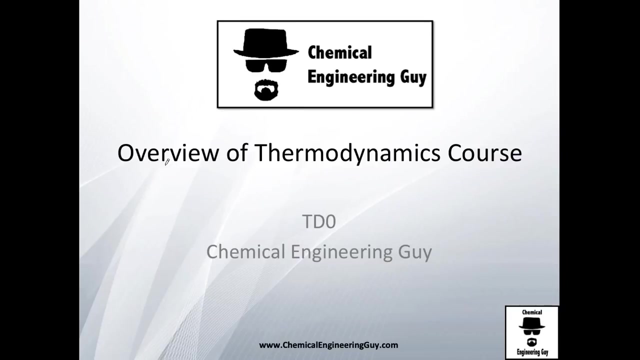 So what's up, guys? I'm very happy that you choose to take the thermodynamics course. I'm going to give you the overview of what we are going to be studying in this course And, as you can see, this is TDO or zero, because it's the beginning, And be sure to check out this site here. 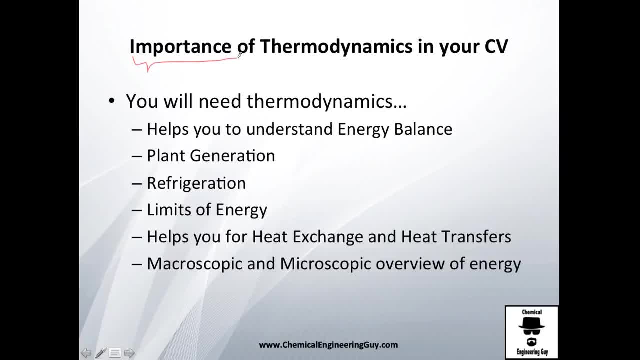 Now, first thing first. why should you study thermodynamics, its importance and why you need it in your curriculum? And the first thing that pops into my mind is because you need to understand it for other energy balances and how heat is exchanged. 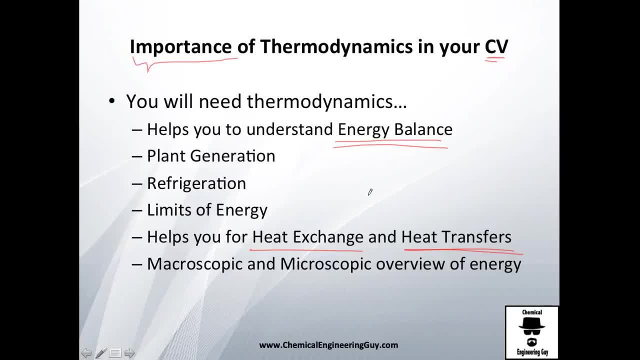 And how the heat is transferred. how can you change heat into mechanical work and that mechanical work maybe even change to electricity, like in the plant generation. We're going to see a little bit on that. Also, it's very important, the refrigeration topic, which is how can we cool a system. 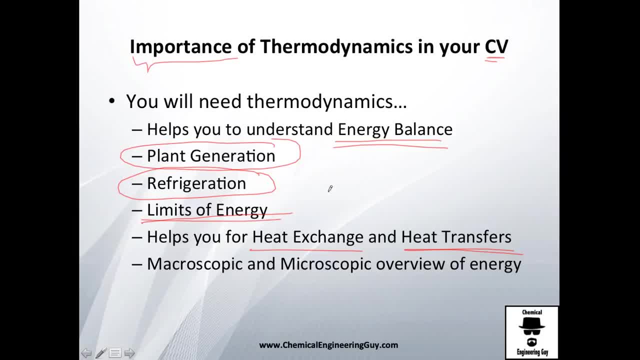 We can then, after this course, understand the limits of energy, or the limits of heat and heat transfer, and also the interaction between work and heat. What else can we see? And we will see a little bit on the microscopic overview of energy, but mainly we're going to see more into the 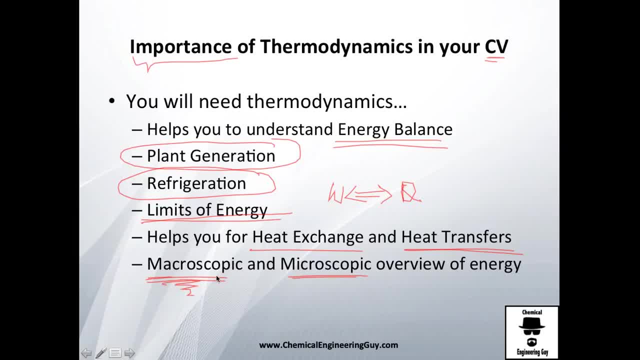 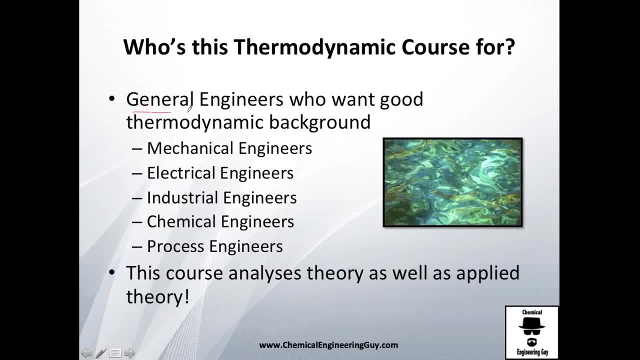 microscopic overview of energy. How can we use that energy? And who's this thermodynamic course for? Probably, I would say it's in general for engineers. I would say it's a very important topic: how to interact with heat. As you can see, we're going to see a lot of people doing a lot of work, but of course it's more into mechanical engineering, electrical engineering, even a little bit with industrial engineering, chemical and process engineering. 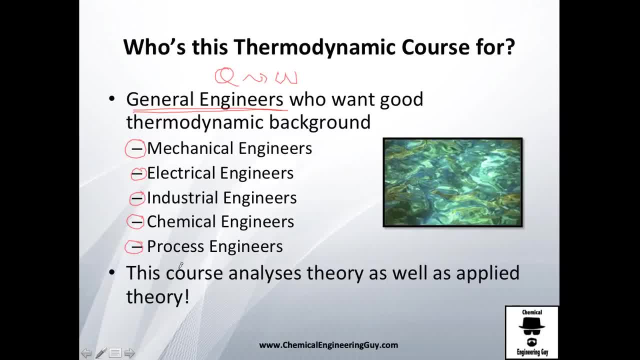 These are the top engineers that will of course take the most advantage on the course. Or if you're in computer engineering or something like that. it might even also help you to know how cheap processors may be cooled and all those kinds of stuff. 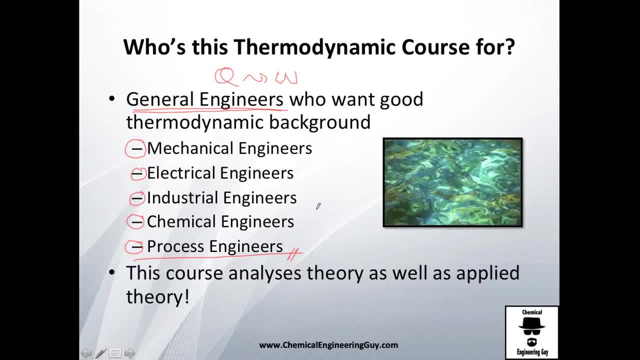 And I'm very happy to tell you that, even though we're going to see a lot of work in the next five years- we're at least going to see a lot of work in the next five years, though we're going to see a lot of theory. the point of the course is to 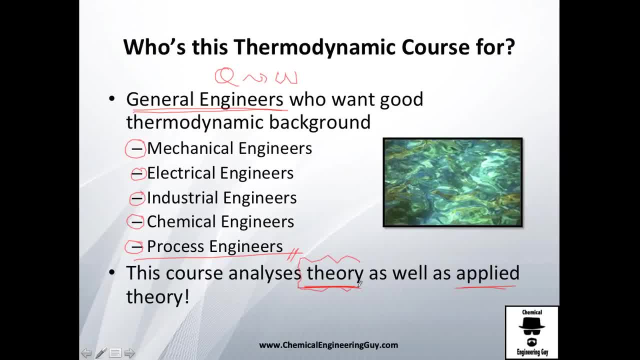 apply that theory, because knowing about a lot of concepts it's okay, but if you don't know how to apply them in real life or in engineering life, I think it's not that worth to know them if you don't know how to apply them. So still, 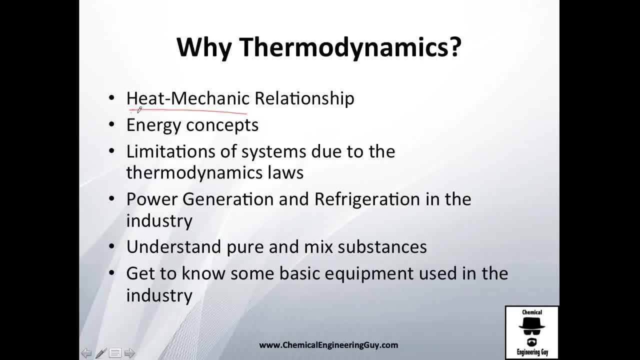 wide thermodynamics. we need to know that heat and mechanical work relationship. many energy concepts- I'm pretty sure you don't know many type of energies that we're going to be studying in this course. also, once again, the limitations due to thermodynamical laws. we have at least four laws: 0, 1, 2 and 3. we need to. 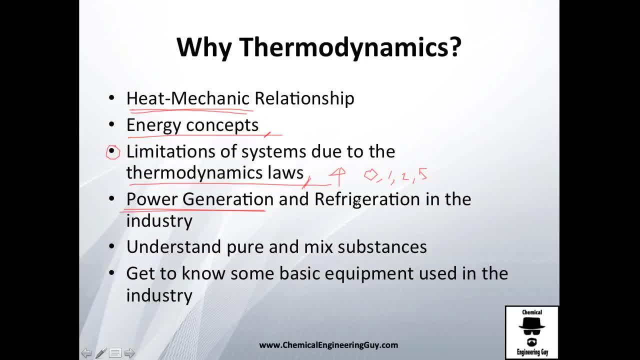 see a lot of power generation, especially electricity, or more how to interact with heat. we can transform it into mechanical work and mechanical work we can transform it to electrical energy and, of course, refrigeration, which is a very important industry, especially in food industry and many other chemical processes that. 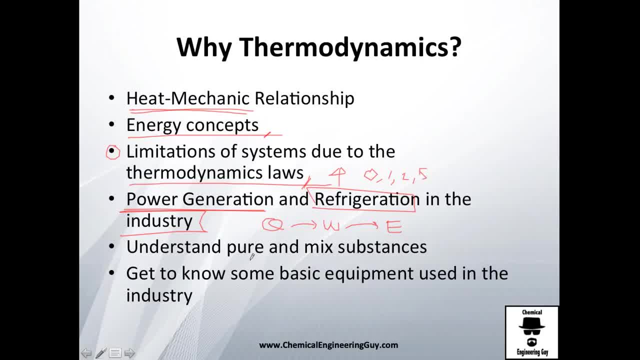 involve having low temperatures and all those kind of processes. also, we need to understand the difference of pure substances and mixed substances and how they interact between each other, And hopefully after the course, you will know the basic equipment that we use in engineering, especially in process engineering, for example, pumps, boilers. 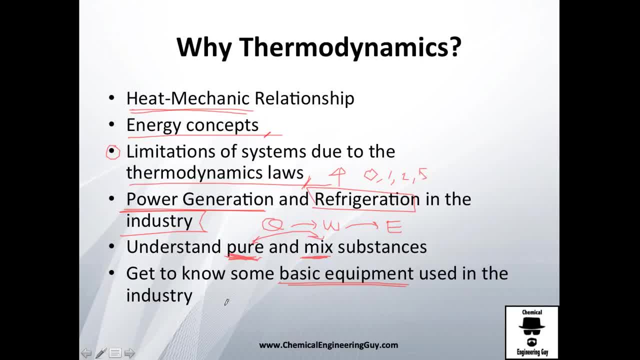 heat exchangers, condensers, all those kind of processes, even turbines, bulbs, many other. we're going to see a lot of equipment and we're going to be analyzing the mass and energy balances of each of these equipments and, of course, how to use them. 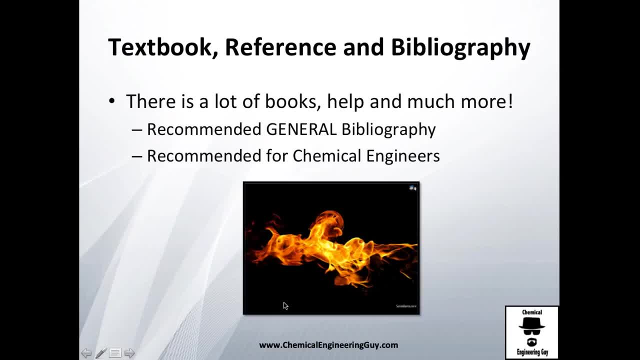 and, of course, how to use them. How do they work? Now, about the textbook that we're going to be using and your reference and all that bibliography you can get. the good thing on thermodynamics is that we got a lot of materials, so that's not the problem. actually, the problem is which one would 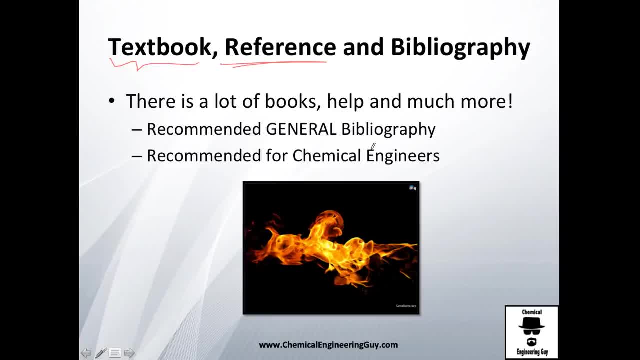 you choose and which one makes more sense, which one is easier to get and which one is more available. I'm going to recommend you your in general engineering- mechanical engineering or even chemical engineering- a general bibliography that I think is pretty good- actually it's my favorite one- and if you're 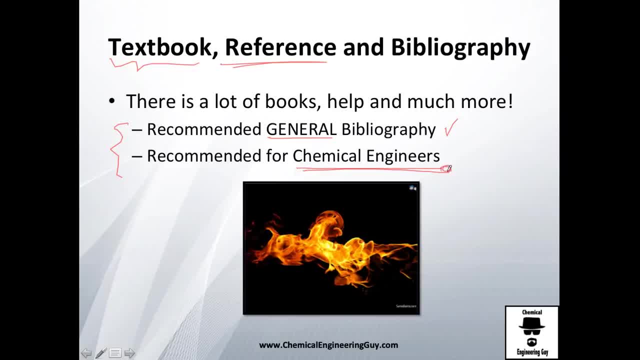 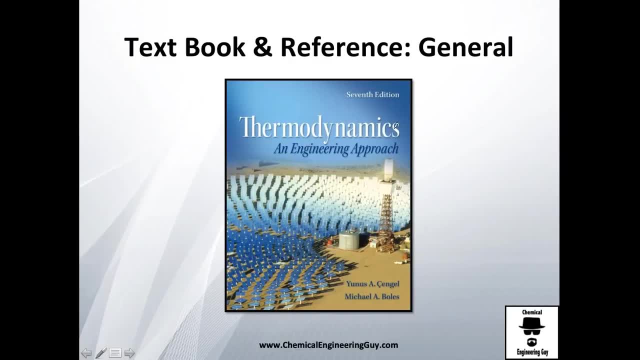 studying chemical engineering. I'm going to give you a little bit more on that. so about the general engineering, I will recommend you definitely this book, which is thermodynamics and an engineering approach, because actually thermodynamics is a science rather than a subject, purely engineering. but it's very 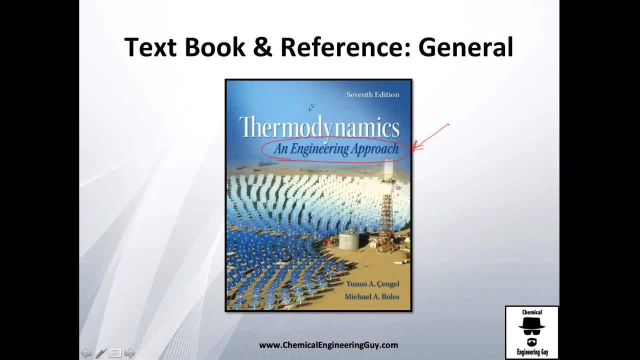 important in process engineering. so that's why these thermodynamics books makes an approach in engineering and it's pretty awesome. I really recommend it. it's actually the- of all the books I've read before on thermodynamics, I think it's the one that makes more sense and it's easier to get and has a lot of. 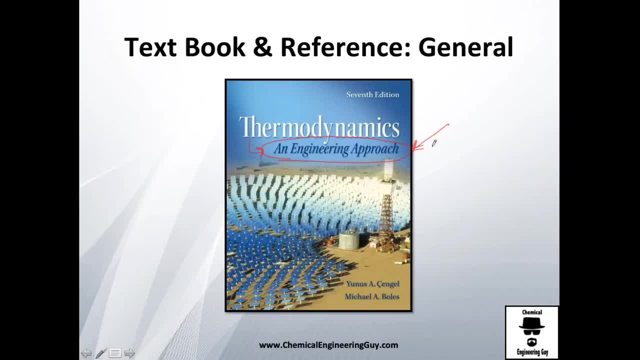 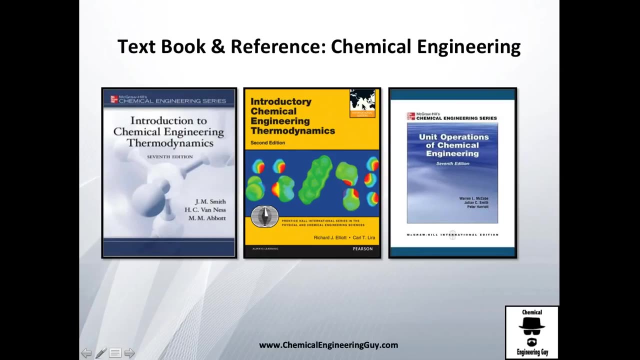 examples and explains you pretty well each of the exercises, and this book is written by Juno Senghel and Michael A Balls. I think there is a eighth edition, but I would recommend you any edition you can get now. if you're studying chemical engineering, probably you will get one of. 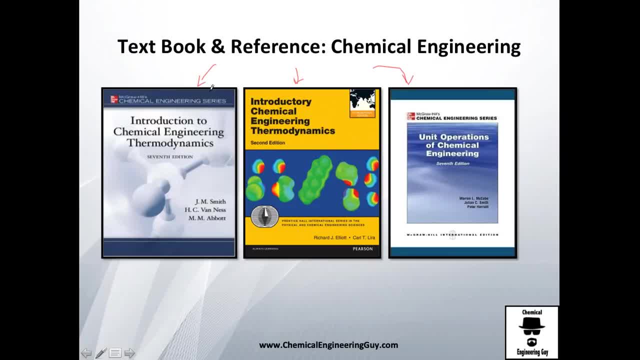 these three books, one of the most typical ones is this one. I really recommend it. if you are then going to study thermodynamics in equilibrium- the introduction to chemical engineering thermodynamics, by Smith, Van Ness and Abbott, I think it's a good book. I think it's good a little bit, I will. I will rank it 4 out of 5 stars. you, I think. 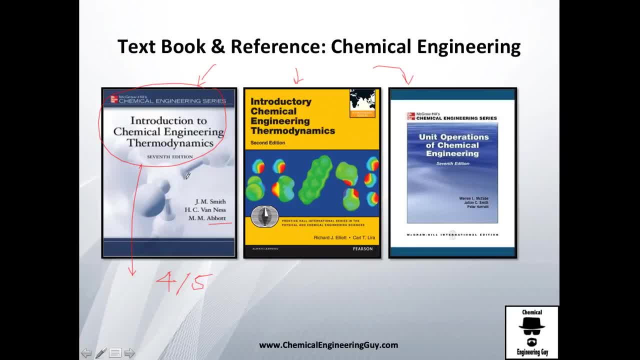 eventually you're going to buy it, so buy it as soon as possible. if you're starting with this course, I will totally recommend you guys now introductory chemical engineering- thermodynamics. I actually haven't read it or use it that much, but what I have been in contact to I don't like it that much because they 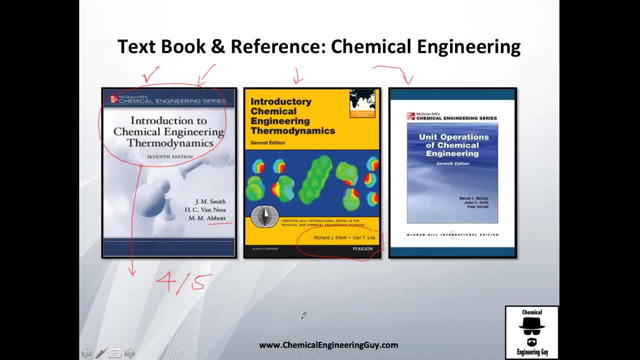 start giving you a lot of abstract concepts and they start studying entropy, which I think is a little bit too soon for that. I would rather start analyzing first law and then I will go to the second law. but they go directly to entropy, I think in the first or second chapter, and it's okay. 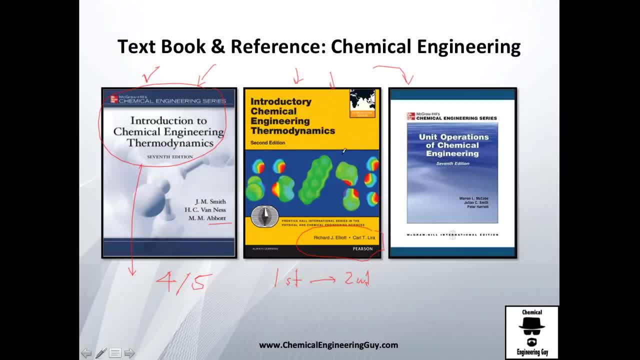 because eventually you're going to stumble upon that. but I will not recommend it that much if you are not a chemical engineer. Actually, as a chemical engineer I will not that recommend it. I will give it maybe two out of five stars personally, even though it's a good book. but 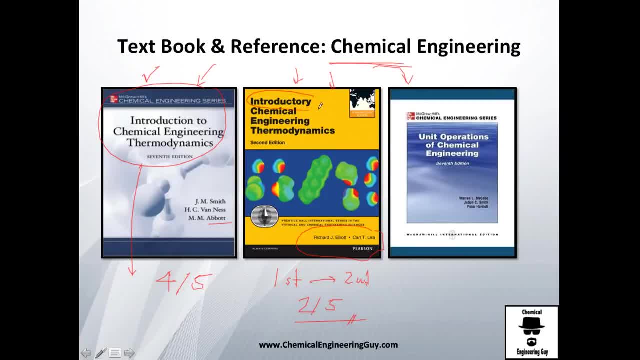 as it means introductory. I don't think so that much. And then you're going to see this book, which is one of the most famous book for unit operations, actually higher, let's say higher- subjects in chemical engineering. It's from McCabe and Smith. It's pretty awesome, but the thermodynamic part is not that into thermodynamics that we need. so 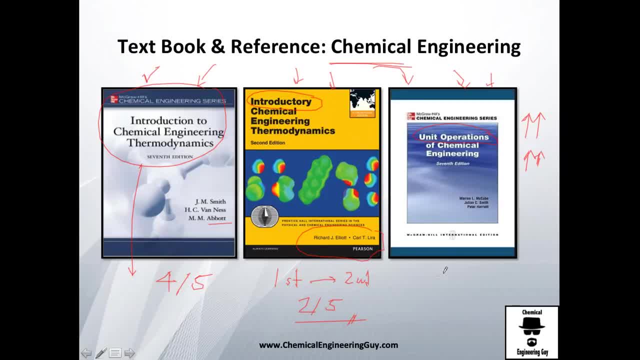 I will not recommend it. I will give it also maybe three out of five stars for thermodynamics, even though for unit operation I will definitely give it five out of five. So it's up to you guys whatever you want to. they cover almost all the topics that we're going to. 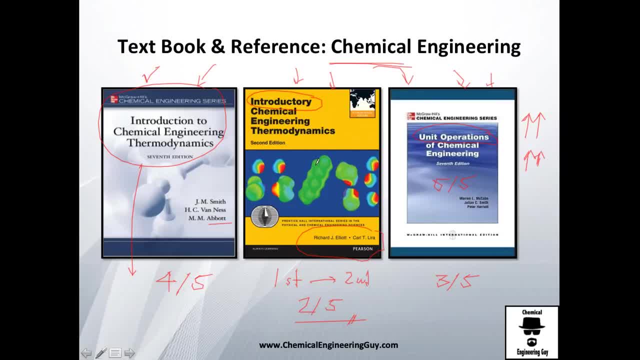 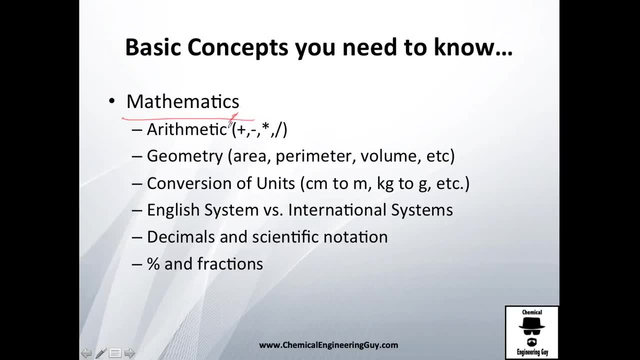 cover in this course. so whatever you can get in your hands, it's good. About the basic concept you need to know before. well, you've probably seen this slide before you know. you need to know a little bit on arithmetics, geometry, for example, how to calculate area. 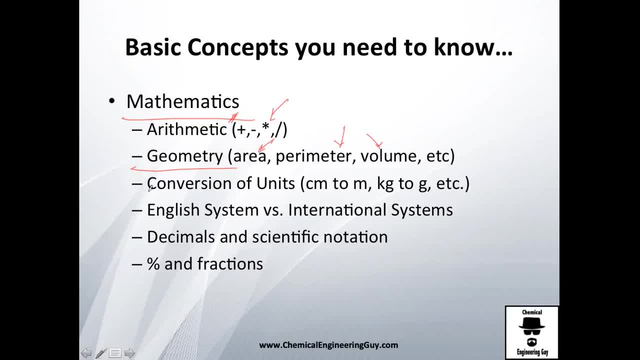 volumes, even perimeter. You need to know how to convert units like centimeters to meters, kilograms to grams, etc. And most importantly- and we're going to practice a lot in this course- is changing from English units To international system units. for example, Fahrenheit to Celsius, BTU, which is British Thermal Unit. 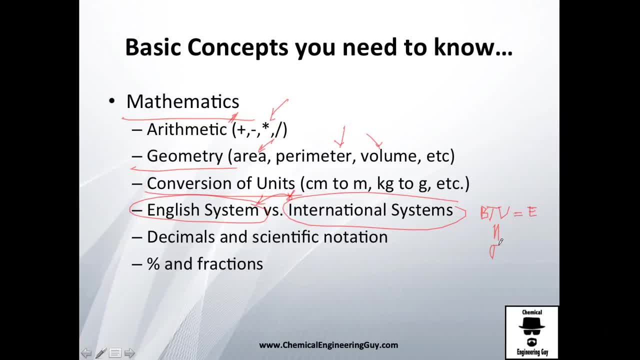 a measurement of energy to joules and all those kind of units that we're going to see in here. Please make sure you at least know the equivalent or you have a table behind you, because it's going to help you a lot. Decimals and scientific notation: this is very important. we're going to work a lot. 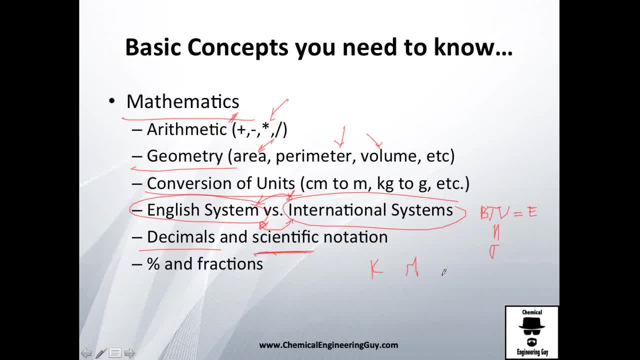 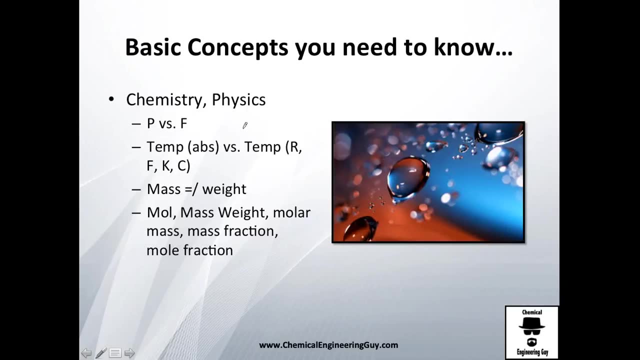 with, For example, Kilo-megas, micro even, etc. And where else, Percentage and fractions. this is important, especially for efficiencies, vapor quality, etc. Now on chemistry and physics. actually, since this is an open thermodynamic course, you don't need to know that much into chemistry. 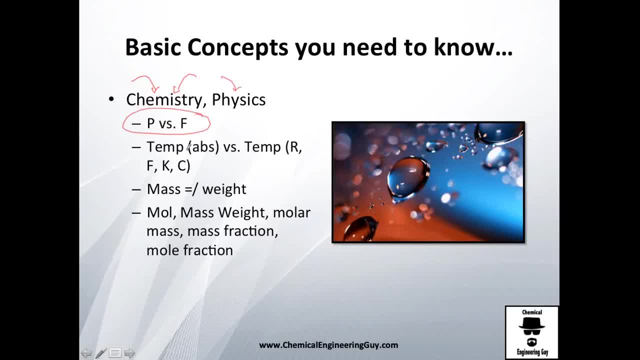 and not that much into physics. I'm going to give you a small review on difference pressure, weight, force, mass, etc. I'm going to give you an overview on the temperatures. also, what's a mole mass weight? how to interact between them. 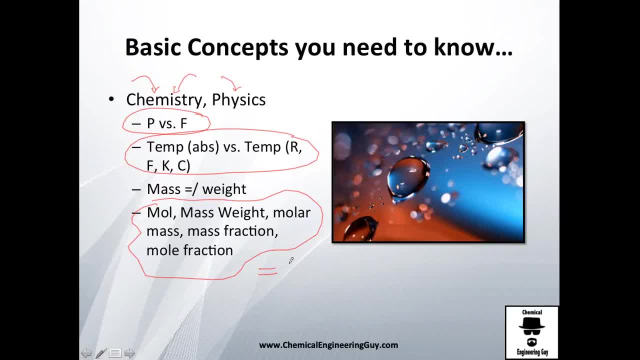 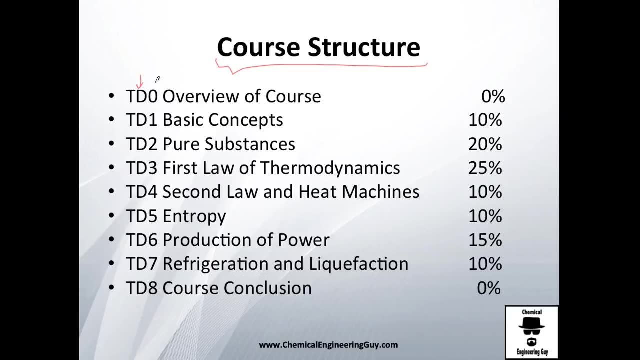 molecular weight, mass fraction, mole fraction, etc. So actually you just need to know a little bit math and the basics on chemistry and physics. Let me give you the course structure here, guys: TD as thermodynamics. I broke it down into eight. let's say like blocks, block number zero and eight of course are 0%. 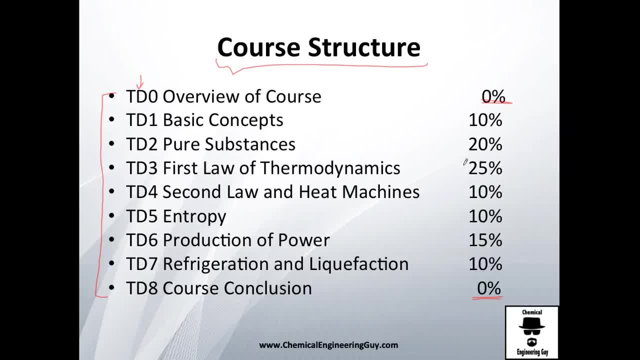 because it's the introduction and the conclusion. As you can see here, the highest one will be TD3, first law of thermodynamics. I think this is the most, one of the most important parts in the course. If you get this, you will get. 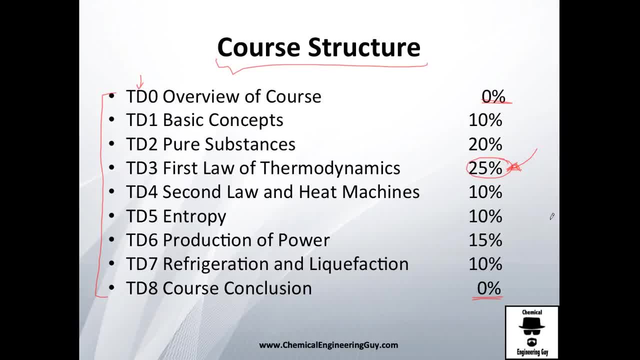 easily. all these, all the other subjects. What else Also, pure substances. this one is very important because if you're going to be studying about substances and thermodynamic equilibriums and mass transfer, heat transfer, etc. in further courses, you are going to use this. 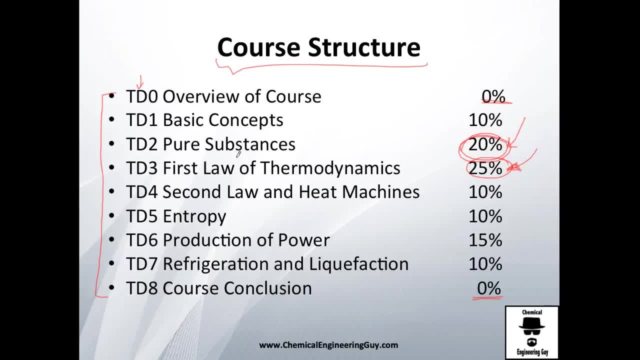 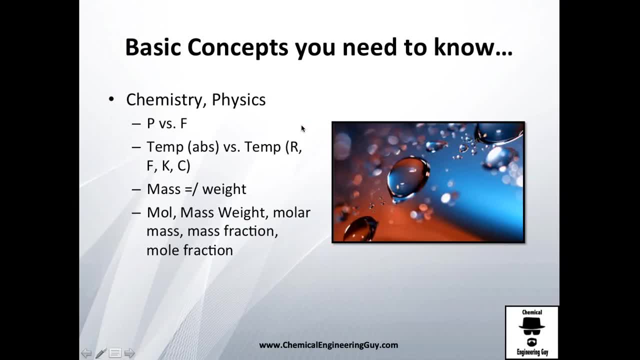 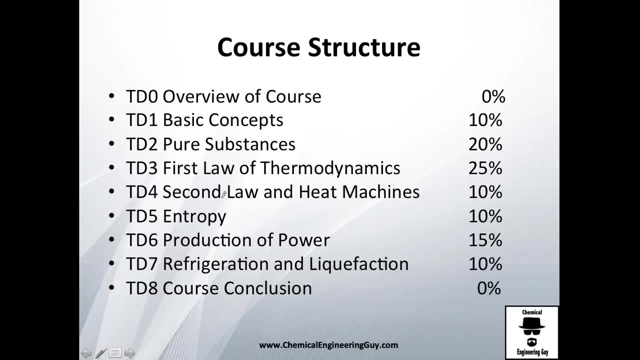 absolutely like. I'm pretty sure you're going to use it and it's very, very important. Basic concepts is the one I'm going to be showing you. all those chemistry and physical concepts. What else do we have here? TD4, second law and heat machines. we start analyzing a. 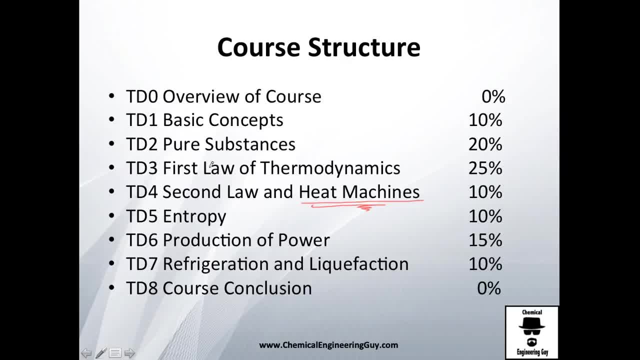 little bit on heat machines. We're going to see the complete course content in the next slides. What else? Production of power: this is also very important, especially for mechanical engineers or electrical engineers. Refrigeration and liquefaction: I think it's also very important, especially for those who want. 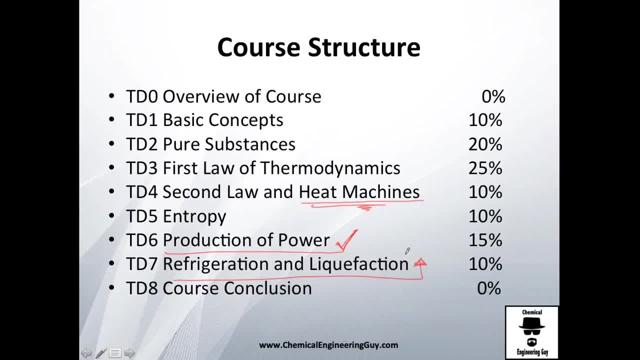 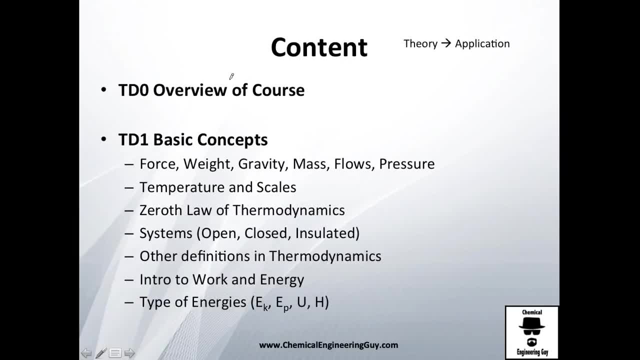 to learn how to cool down systems in the most efficient way. And finally, we make the conclusion. And as I told you before, guys, this is the complete content, or at least a more in-depth content. We're going to be analyzing theory and then application of that theory, So don't think that we're 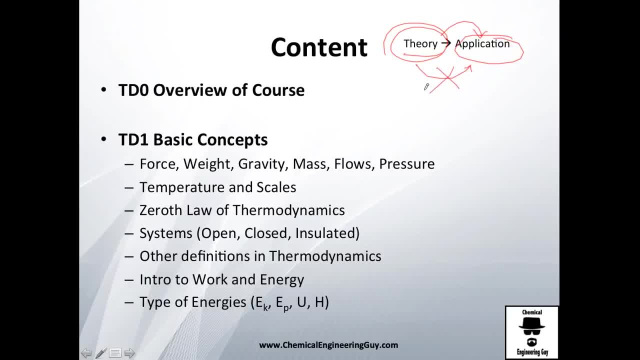 going to see a lot of abstract things and never apply them. no, We're going to see, maybe, abstract things and then we apply it as soon as possible. so you get the idea and why is it important to study that? So we start with basic concepts, as I told you before: force, weight, gravity, mass. 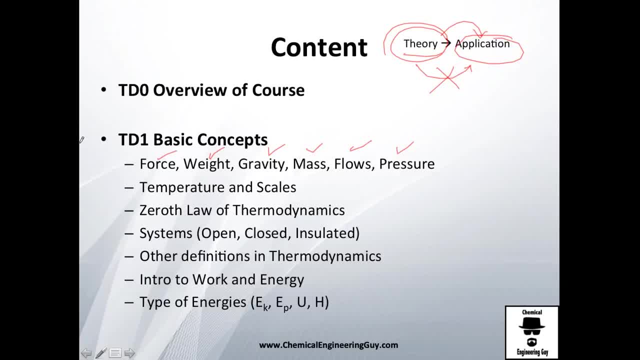 flows. I want you to get them completely like perfectly definitions of that. I want you to be doubt or free of doubt there. Then we start with temperature, the difference between temperature and heat and, of course, the scales we have there, The serial law of thermodynamics, which is actually pretty simple, The type, 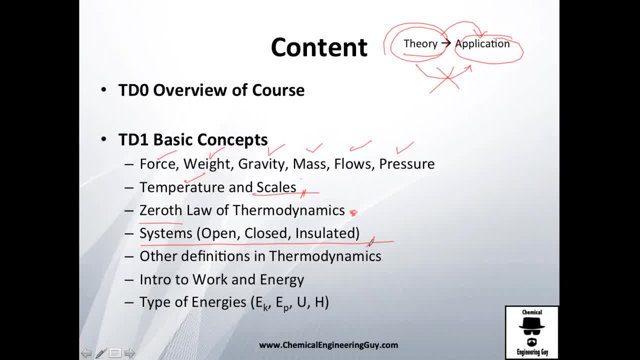 of systems that we are going to be analyzing: open, closed, insulated and isolated, etc. Many other definitions that maybe are easy to- or at least you've been talking about that, but not that- into the most technical terms. And then we continue with the relationship between work and energy. You might think. 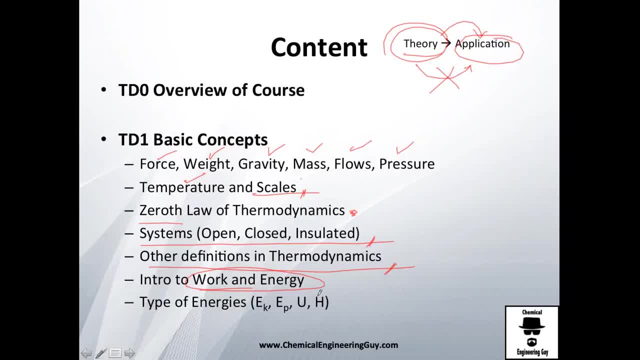 they are the same but they are not the same. They are similar but not the same. And since we will be talking about energy, why not introduce you to one of the most typical type of energies we're going to be finding in the industry, which is kinetic energy, potential energy, internal. 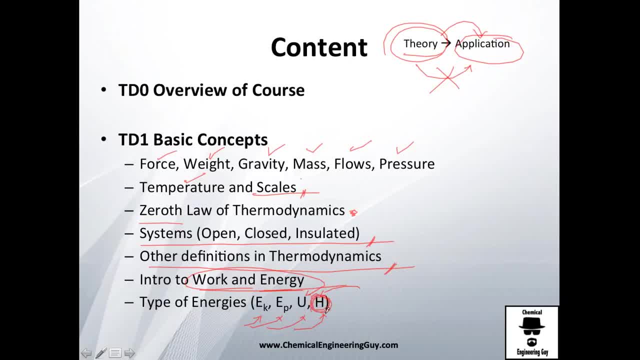 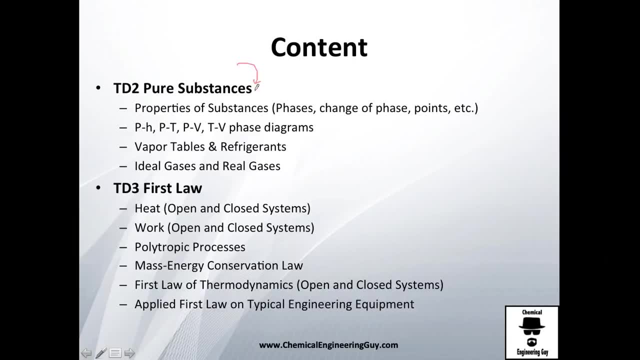 energy and enthalpy. This one is a special case. Good, once we get those basic concepts, we can jump to the second block, which is TD2, pure substances. We're going to analyze properties of the substances, how or what is a phase? how do 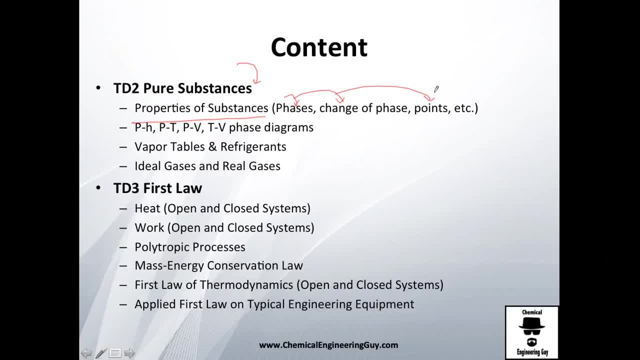 they change between them all the important points, such as critical point, or all those points, the triple point, etc. Phase diagrams- and we're going to see and analyze a lot of them- Pressure, temperature, volume and a lot of interaction. Vapor tables and refrigerants, Ideal gases- you've probably 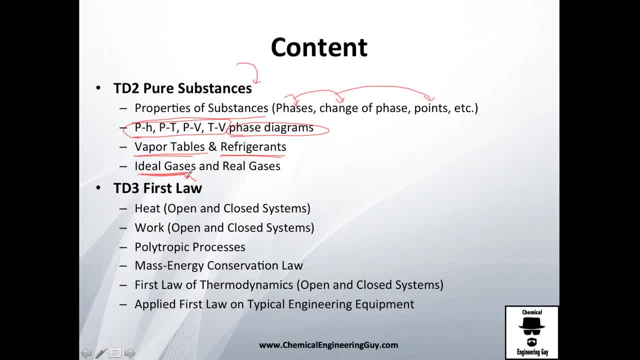 been working with these before, but we're going to give a little insight, just to say that we covered that, And then we're going to analyze real gases. This one is a pretty awesome course. Actually, you might even make a course on that, but we're going to see, of course, just an overview. Then we jump to once we 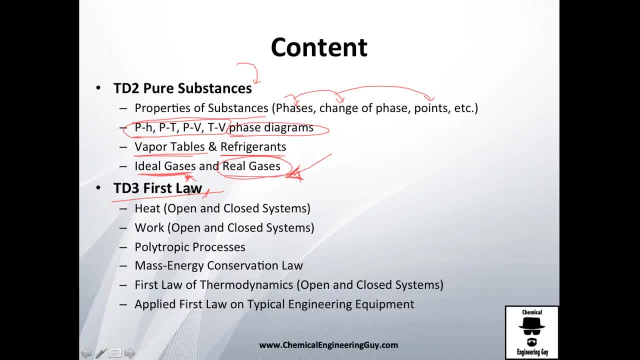 know how substances work and interact between each other. we can jump to the first law. We're going to review heat and work for open and closed systems. Then we are going to see the typical processes or polytrophic processes, such as isobaric, isothermal, isovolumetric, adiabatic, etc. All those we're going to. 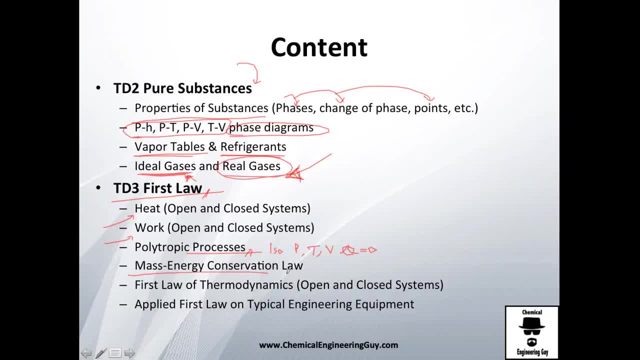 analyze them, We're going to see the relationship between mass and energy conservation. Then we see the first law of thermodynamics for open and closed systems, Once we get, of course, heat work and some polytrophic processes. And then, once we get that, we're going to make a 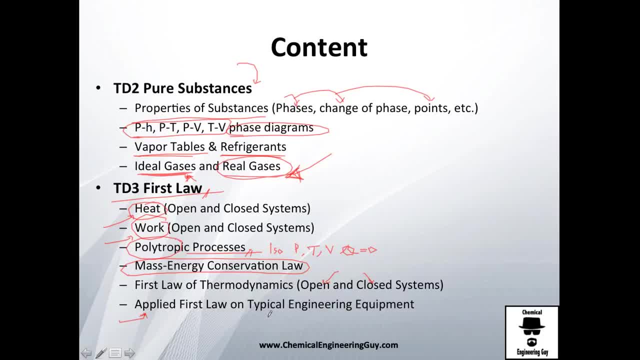 lot of exercise and then we apply it to many typical engineering equipment, such as turbine, a pump, a compressor, a condenser, boiler, heat exchanger, etc. All those equipments that we use a lot in the industry. we're going to keep them the 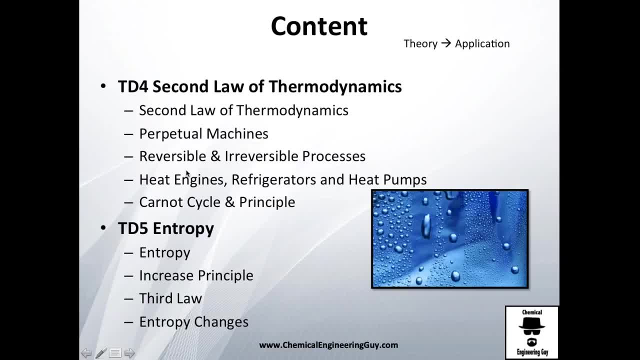 let's say we're going to apply the first line to that. Then we continue with the second law, which is TD4, the second law of thermodynamics. We're going to see what's a perpetual machine as a concept: reversible versus irreversible processes. 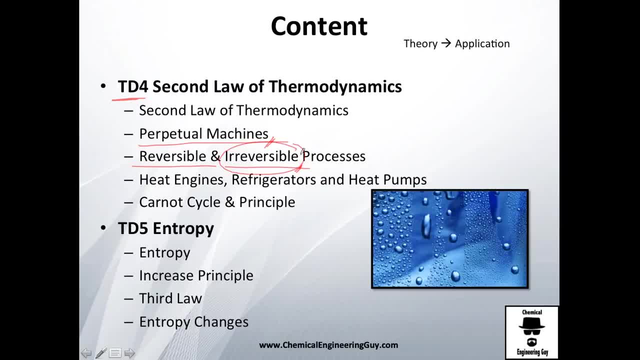 You're going to see that eventually this is not possible to achieve in real life. The heat engine, refrigerators and heat pumps- those are very important. But more importantly, we're going to see the Carnot cycle and the deduction or principles that we can get from there. 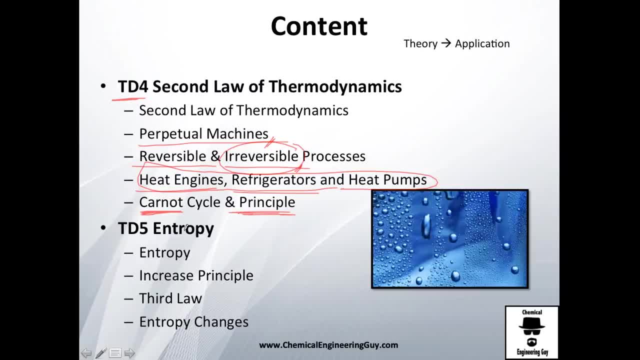 And when we study this, we're going to eventually get into the definition of entropy, which is a very abstract concept. But the good thing is, even though you don't know what's exactly that, you just need to know that if entropy increases, then this is possible and therefore you will be able. 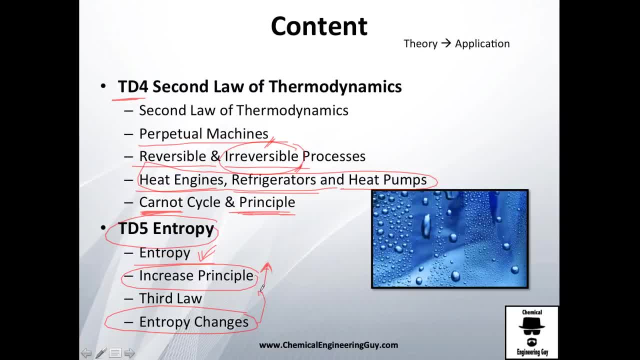 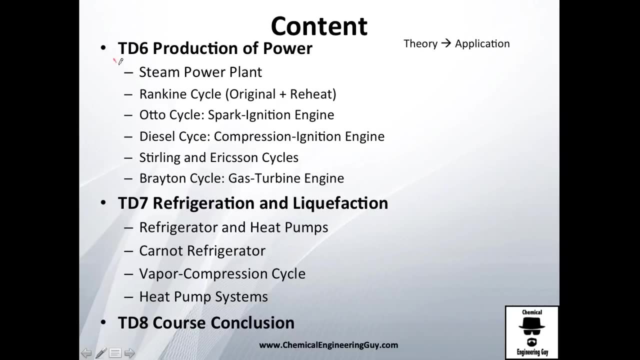 to be calculating those changes on entropy and know if the process might or may not be achieved. And eventually you need to know also the third law, which is a pretty simple law but very, very important and powerful law. And once we know a lot of theory or theoretical concepts, we can actually start applying. 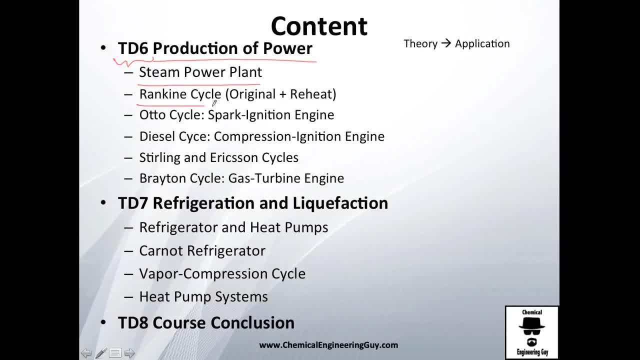 to production plants, For example, the steam power plant ranking cycle, the original cycle, or including the red heat cycle, auto cycle, which is the one with the spark ignition engine, diesel cycle. probably you know it because it is in a lot of motors or engines right now. 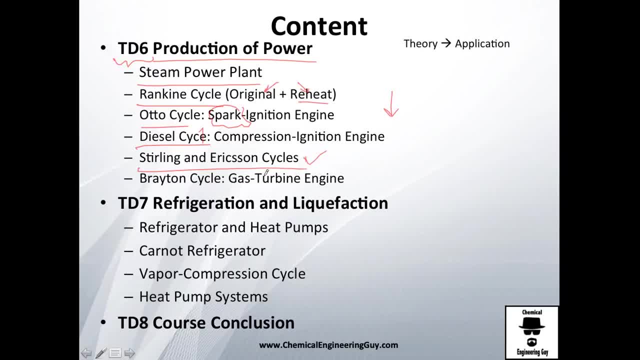 Stirling and Erickson cycles- a little bit overview on that- and the Brayton cycle. Good, that's about generating power. but what do you? what if you want to cool something you know are not interesting in generating power but consuming that power into refrigeration? 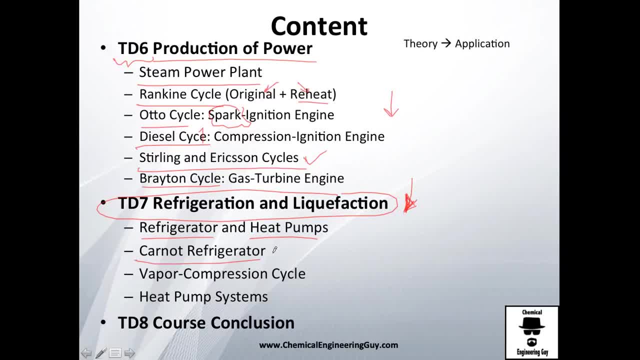 We're going to see refrigerator, heat pumps, the Carnot refrigerator and the vapor compression cycle, which is the real one, because you know Carnot- you will see later that this is more theoretical, this is the real one- And heat pump, which is kind of similar but it is not a refrigerator. And, last but not, 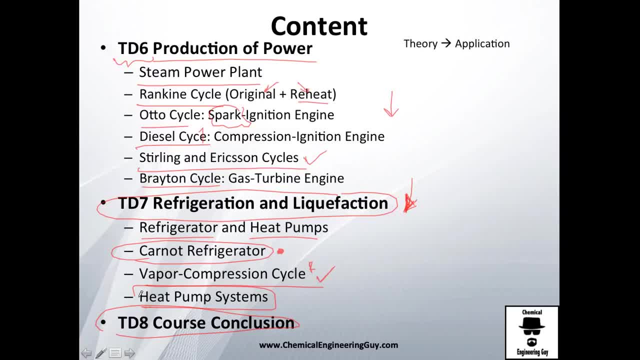 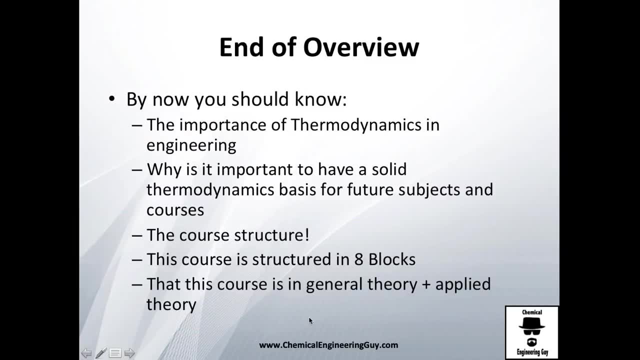 least we make a small conclusion on what we've seen. what do you need for the next courses and what you should have learned? And this was the end of the overview. guys, I'm very happy that you got everything here, and by now you should know the importance of thermodynamics. 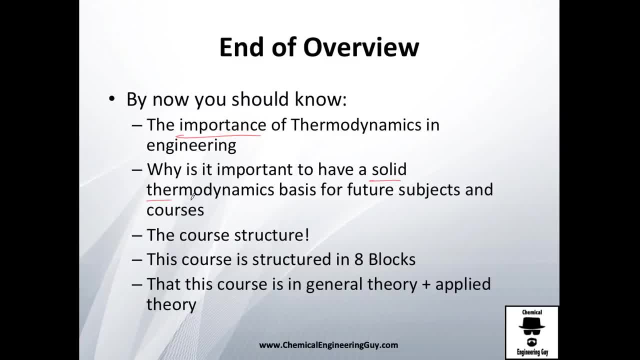 and why do you need to have a solid thermodynamic basis, not only for this topic, but for subject or future subjects or courses. You know the course structure, so if this is very important, guys, so you know why you're studying that first and that after. 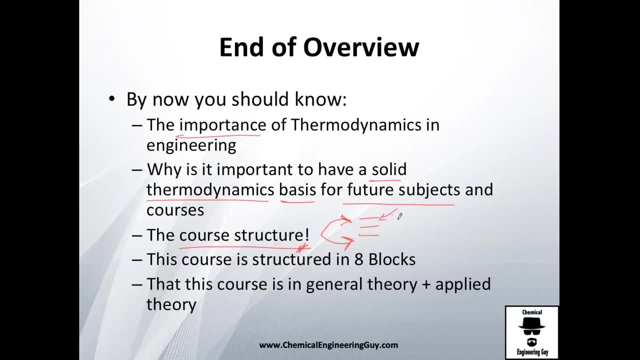 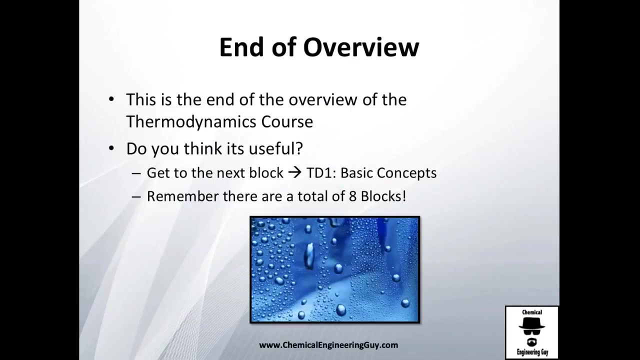 Thank you for watching. Please note that there are eight blocks to our introduction and conclusion and six are theoretical blocks, And this course is theory and application on theory, And I think that's everything, guys. I'm pretty sure that you're going to make it, and thank you for joining the course. See you in the next videos.